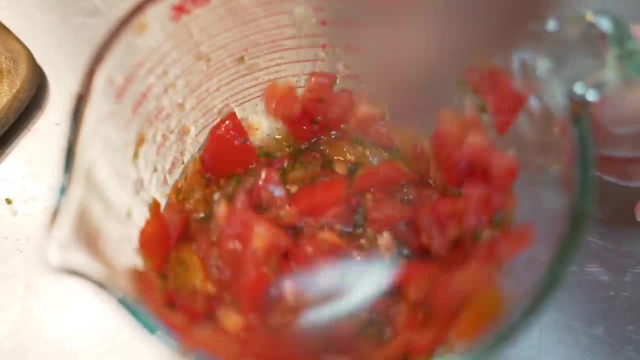 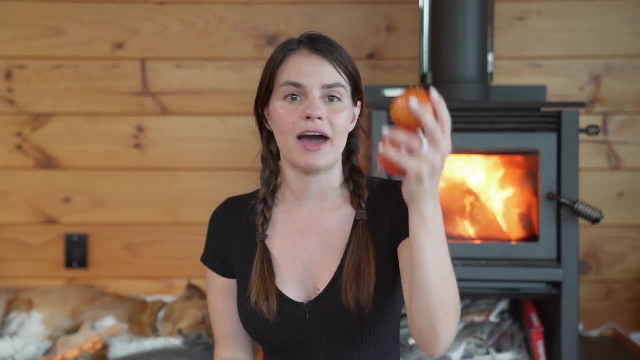 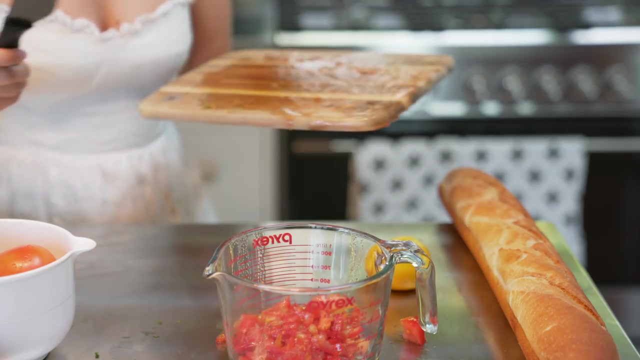 because they are used in so many different recipes. Also, there's nothing like looking out to a green garden and seeing big, red, vibrant tomatoes hanging there, And then you harvest them, bring them into your kitchen, open them up and they're just so juicy. 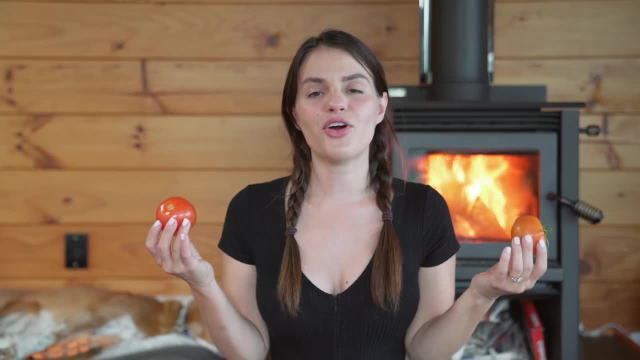 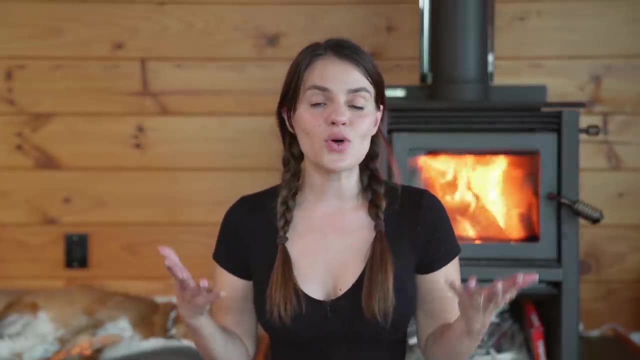 And you're proud of yourself because you created that juice. Well, Mother Earth really did most of the work, but the tomatoes wouldn't have been there if you didn't decide to plant them and care for them. The big questions when choosing to put tomatoes in your vegetable. 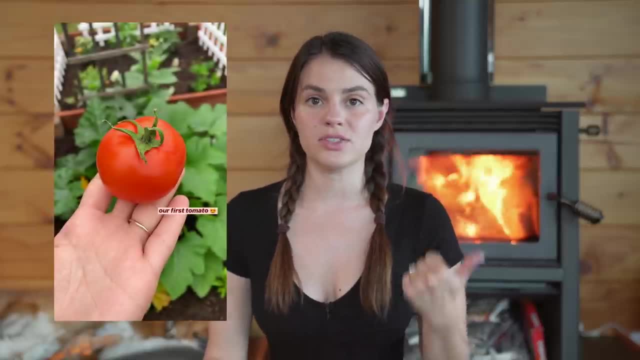 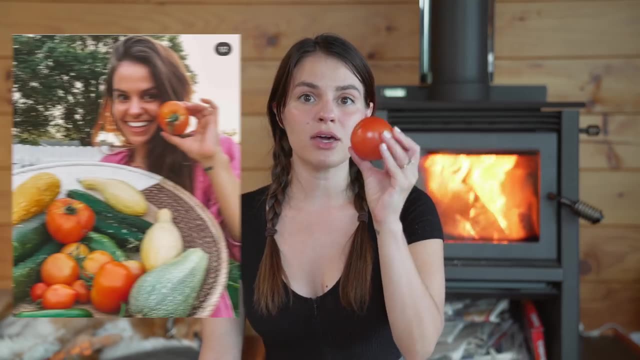 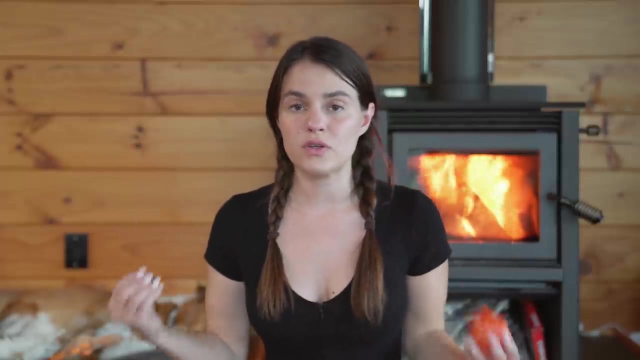 garden are: one, how many tomato plants should I grow? And two, what varieties should I have in my garden? Personally, I love a big Roma tomato And I also really love a cherry tomato. I love having both of those varieties because they can be used for different recipes. 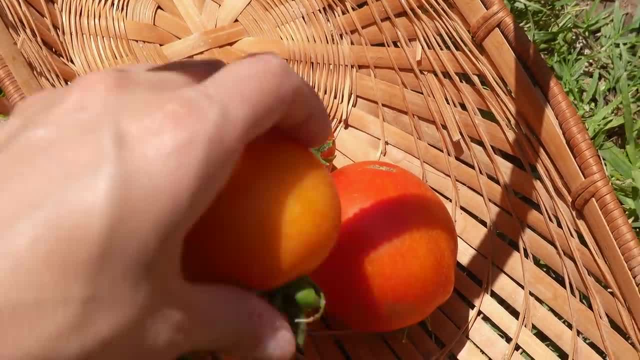 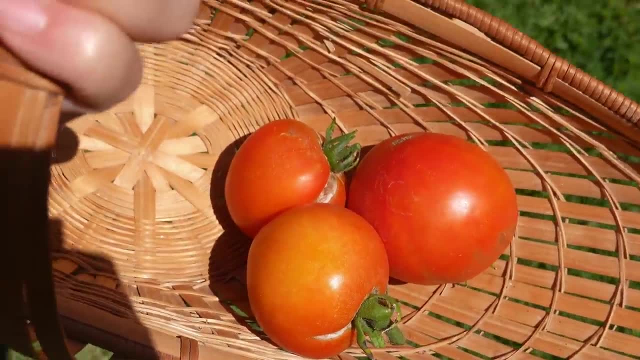 When it comes to choosing how many tomato plants you have growing in your vegetable garden, you really need to think about how many people you have in your household, how often you cook from home and how much you actually like tomatoes, For instance, Alex. and I. we are two people. We have four tomato plants: regular Roma tomato and about two cherry tomatoes. We have three tomato plants and that's been perfect for us. We cook from home on a daily basis and we love putting tomato into our recipes and our meals. 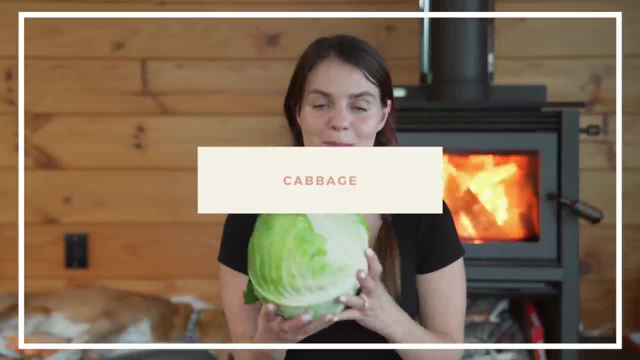 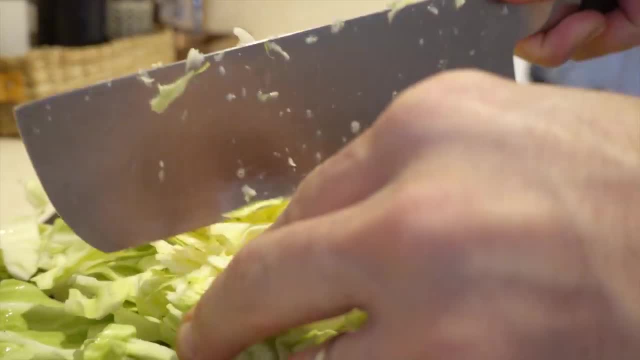 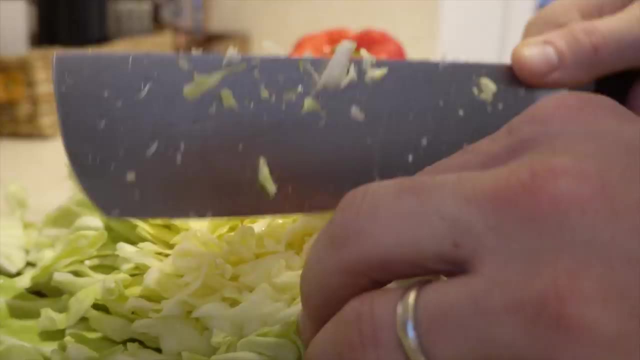 My next vegetable is maybe a not so obvious one, but probably my absolute favorite vegetable that I have growing in my garden, And I never thought that cabbage would have such a special place in my heart until I started a vegetable garden. Not only is it a big, confident plant. 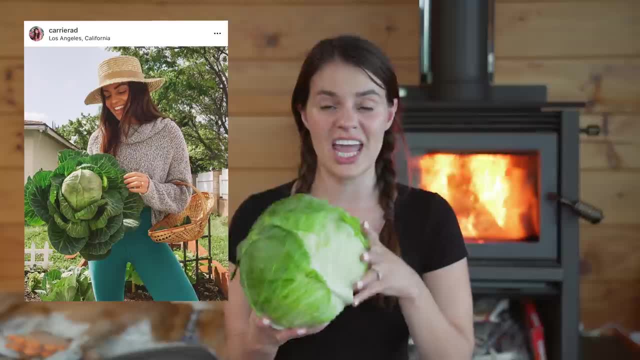 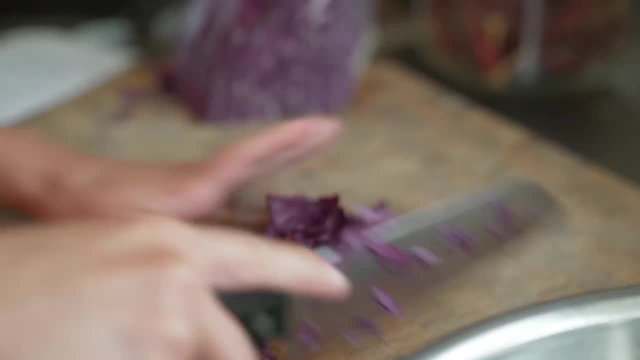 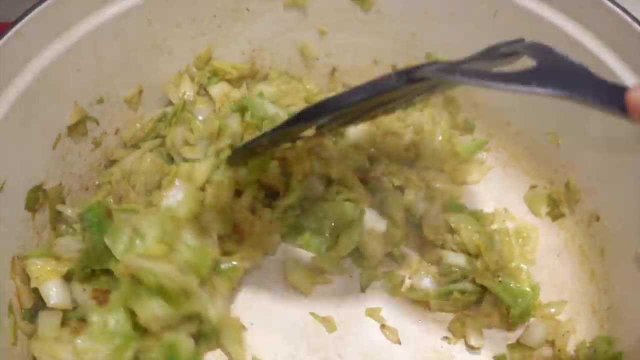 but it also has a lot of nutrients. When you walk out to your vegetable garden and see a veggie this big that you grew from nothing. there are also so many different recipes that you can create using cabbage. It's actually quite delicious in a casserole. You can substitute. 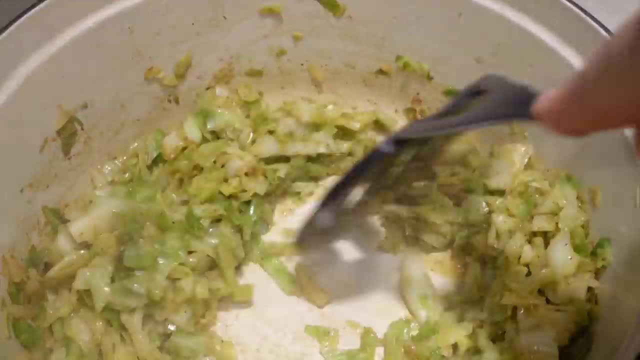 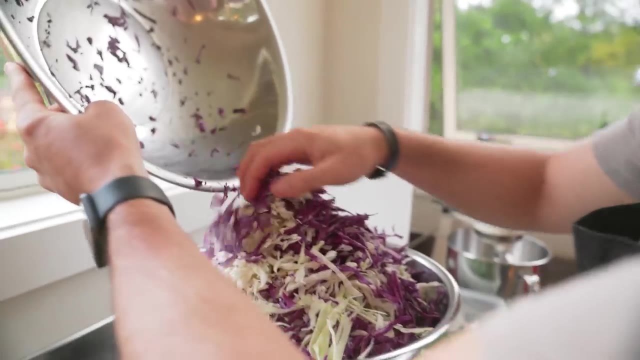 the noodles and add in cabbage and the cabbage gets really moist and noodle-like. And the beauty is you can use the entire cabbage plant in recipes. You can make stuffed cabbage leaves with the leaves of the cabbage. And another thing I love about cabbage is that it will. 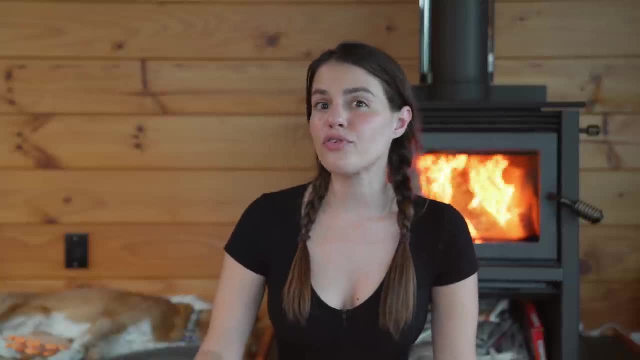 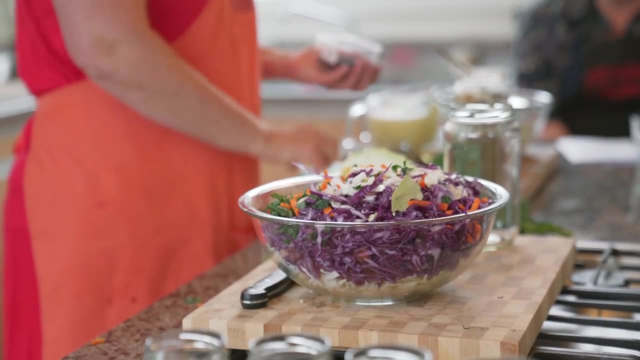 grow in colder climates, So through the fall it will do just fine. When we were living in California we had cabbage go for a couple of years. It never died off on us because we never had a frost And I know in areas where there's a frost it can be a little. 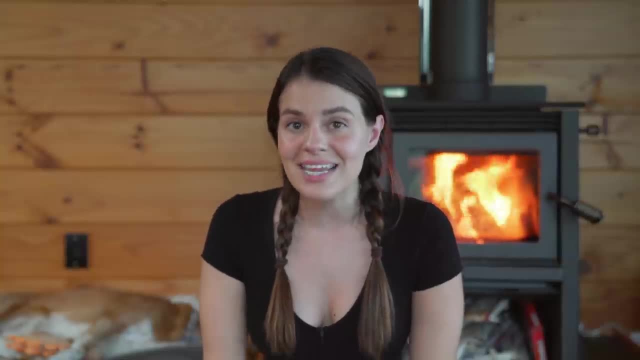 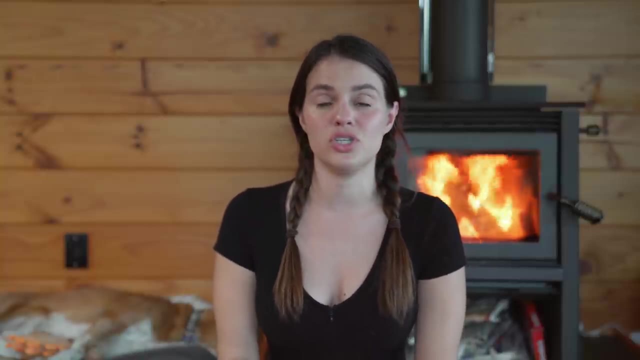 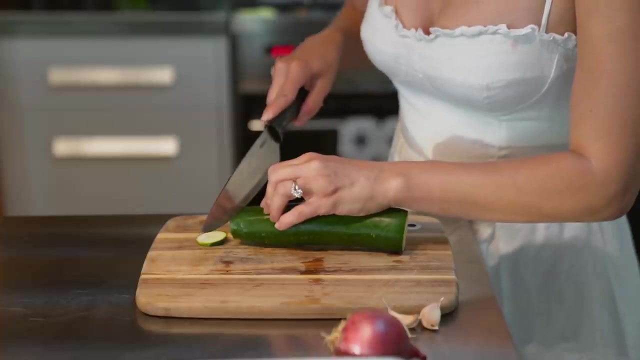 bit more difficult, but your cabbage will last and will do well if you are someone living in a colder climate. This is an excellent vegetable, Excellent crop, to begin with. The next veggie I want to talk about is zucchini. Zucchini is a special vegetable to grow and you have to really pay attention to how you are growing. 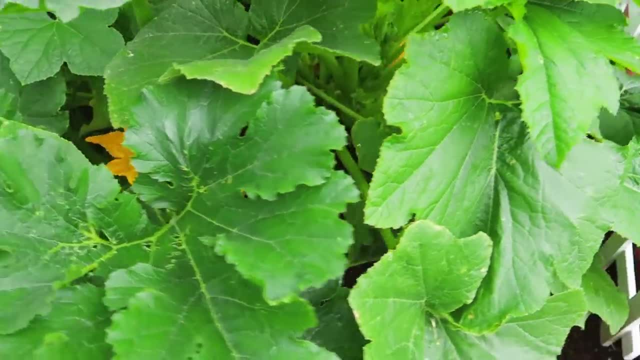 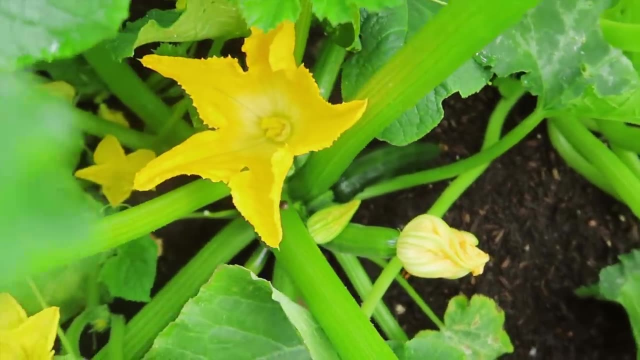 zucchini, because you do not want to have too many zucchini plants. Alex and I, as beginner gardeners, bought a bunch of zucchini sprouts. I think the market that we went to just had a bunch of them. so we were like, oh, why not throw in a bunch of them? We planted them. 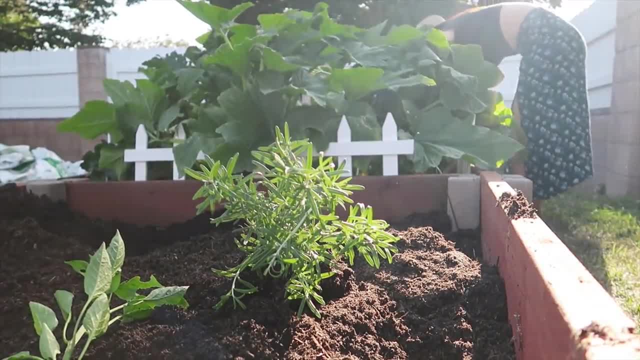 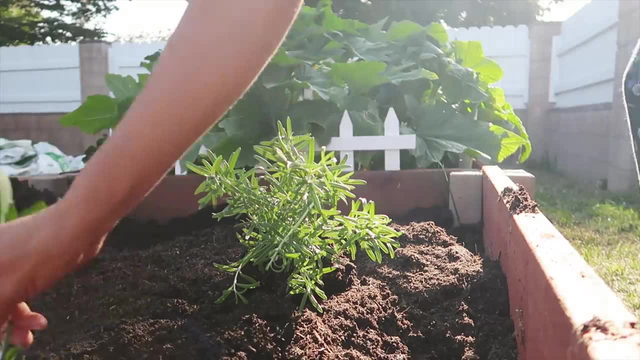 and we had way, way too many, way too many zucchinis growing. We had to give them to everybody. we knew They were all sorts of sizes in our garden. We were so excited, because it's just always exciting when you have an abundant amount of anything. 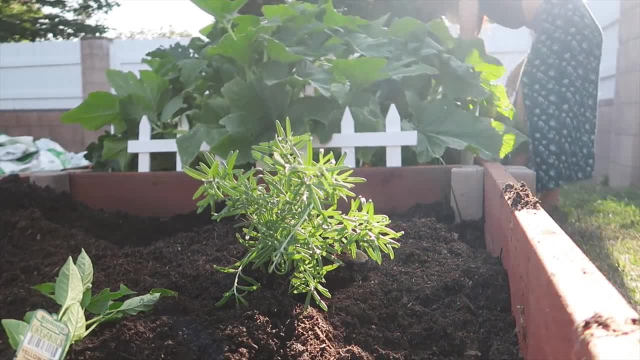 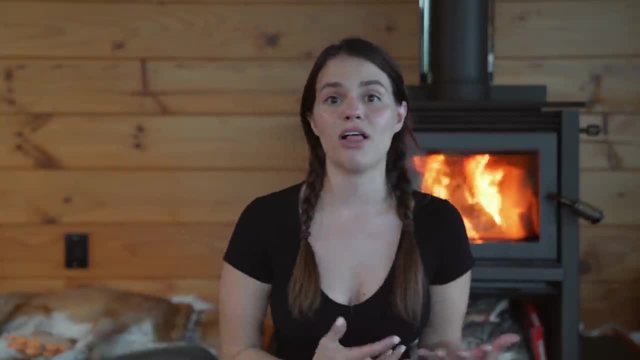 but it also can be a bit daunting when you're trying to figure out exactly what to do with everything. Some of the recipes that I love with zucchini are things like zucchini bread. If you guys were following me during quarantine, I was making tons of different zucchini breads. 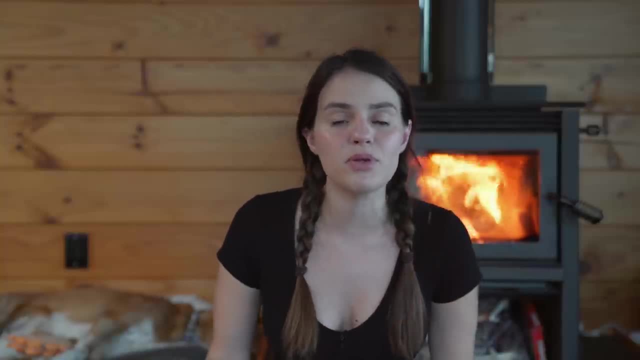 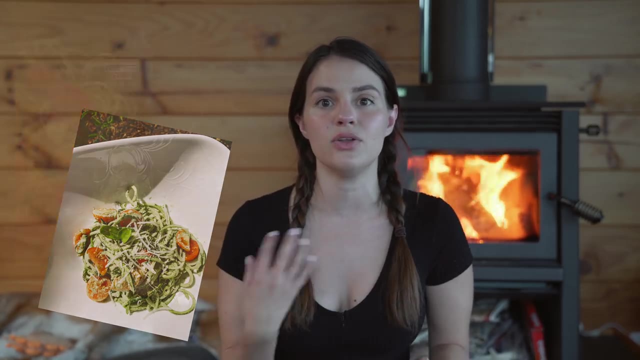 chocolate chip banana bread like cinnamon zucchini bread. that's beautiful in the fall and winter. I also really love doing zucchini noodles and doing like a pesto zucchini noodle pasta, which is amazing. You can put zucchini in a roasted vegetable salad. 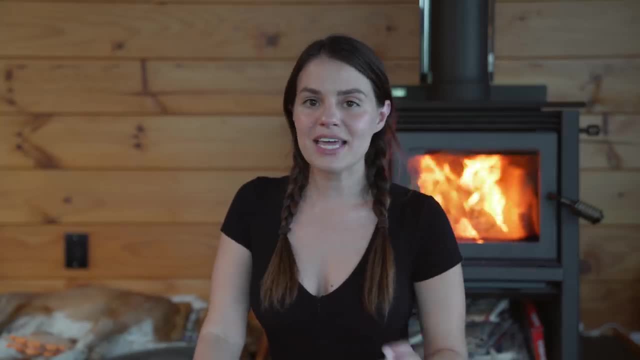 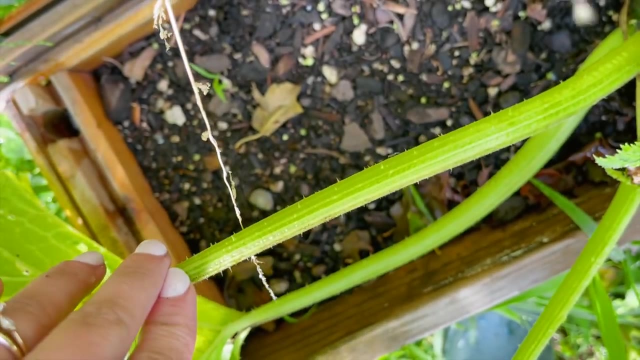 with quinoa. An additional tip: with zucchini, make sure that you wear gloves when you're working with them, when you're cutting off dead leaves, even harvesting a zucchini, because they are, they are an angry plant. I guess you could say: 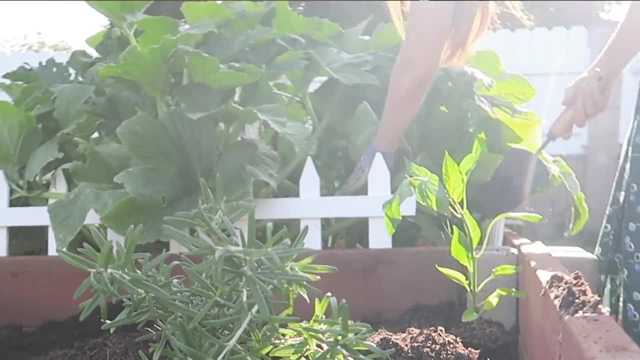 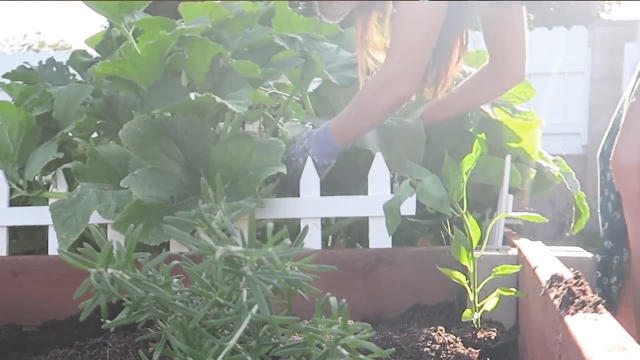 I got so many scrapes and just super itchy skin from working with my zucchini. I can be pretty impatient and I'll be like I don't need. I don't need gloves, I can just go in for it, And I always regret that decision. 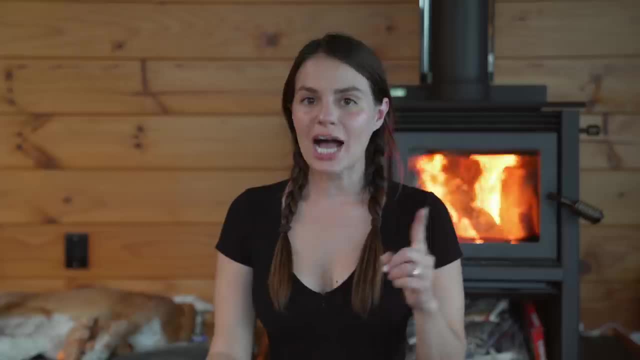 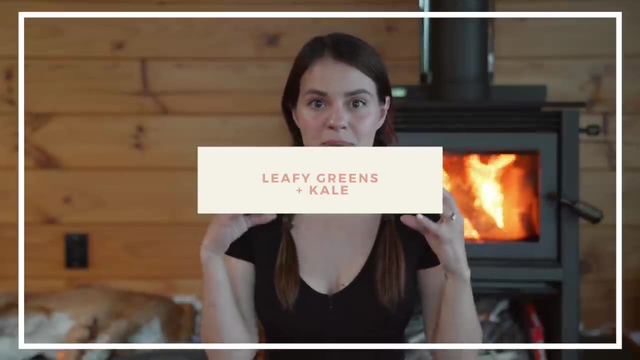 because I end up itchy for a couple of days afterwards. I'm going to cheat for my next vegetable because I'm going to put leafy lettuce and kale in the same category, And I'm doing this because they're pretty much a leafy green right. 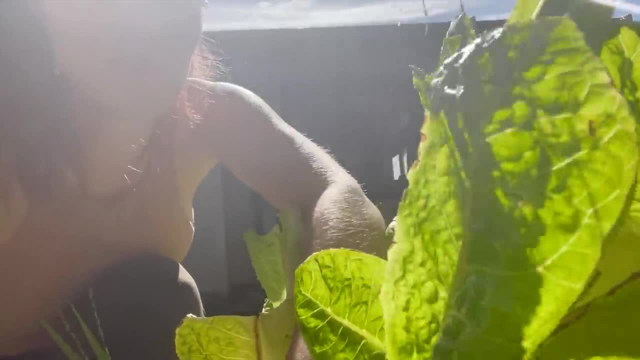 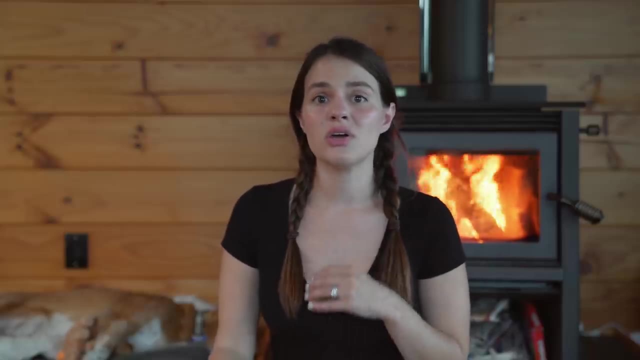 But they actually are quite different. in the garden, Leafy greens like your romaine lettuce can be a little bit more fickle than kale. Kale hardy- It will last years, especially if you are living in an area that doesn't have frost. 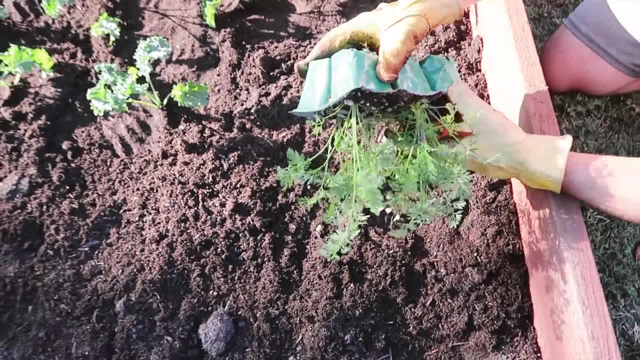 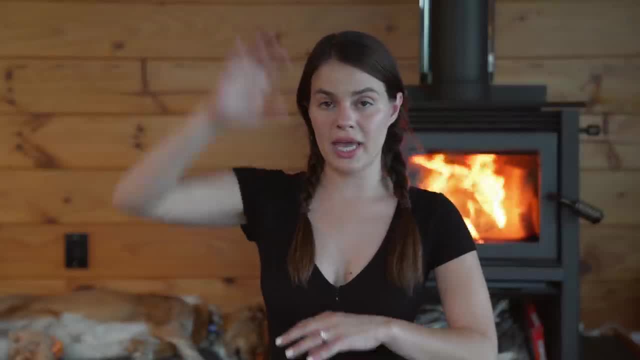 In California we essentially had kale going all year long, and we might be able to pull that off here. in New Zealand too. Kale almost turns into I don't know- a plant. right, It grows into a tree, It grows upward and the stalk becomes super thick. 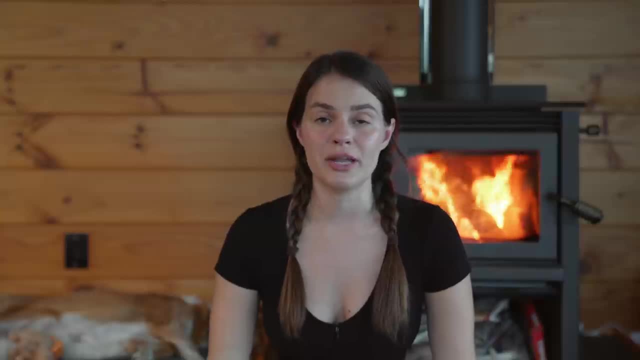 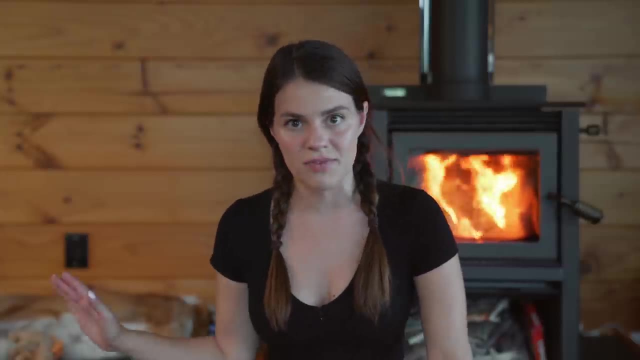 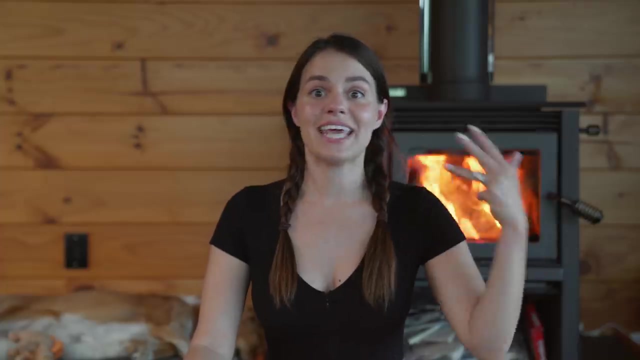 It's really hardy and such a beautiful thing to have in your garden, because it is truly a very easy leafy green to grow And you can use kale for so many different things. Kale is also wonderfully good for you. It has vitamin A, vitamin B, vitamin C, vitamin K. 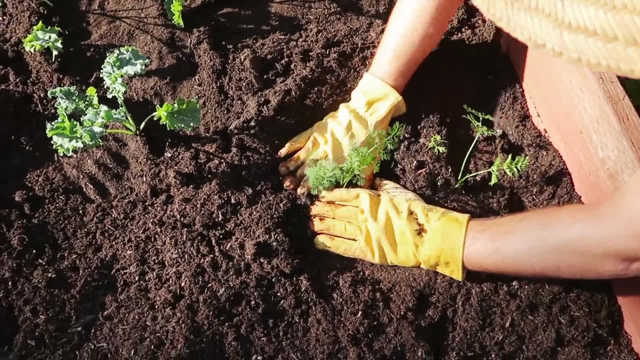 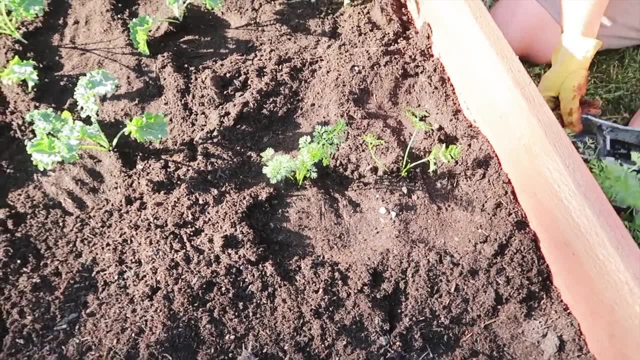 So pretty much the whole alphabet of vitamins. The only thing I would say- an additional tip when it comes to kale, is that aphids love kale. So aphids are these little tiny bugs that live on the backside of the kale. They kind of like burrow into the kale. 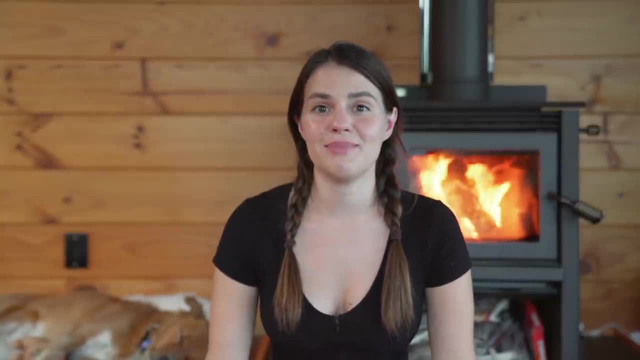 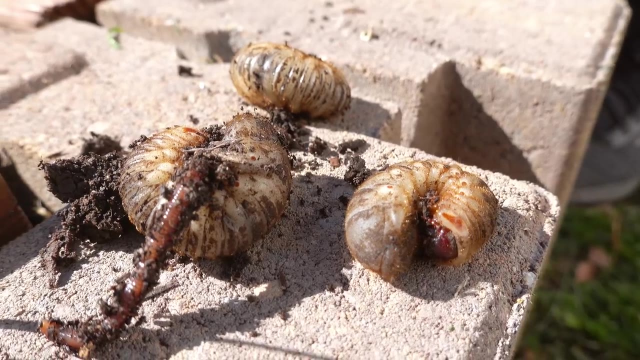 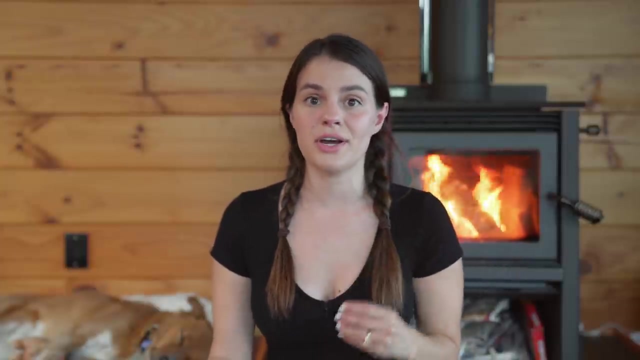 If you don't like bugs, this is probably the hard part of gardening, because they do exist in your garden, especially if you want to grow organically and without using any chemical pesticide. I do have a homemade pesticide. that's really easy to do and it works wonders on your garden, especially kale. 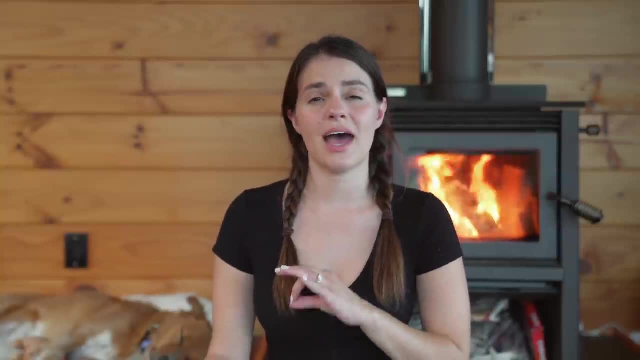 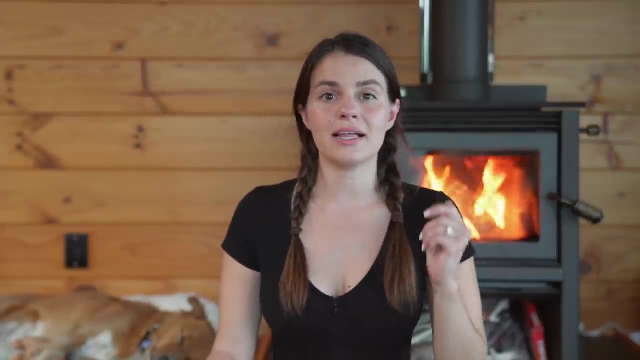 I've had a lot of aphids. We use that homemade pesticide and it actually helped so much. So you can go to my Instagram- It's at Keri Rad. You can go to my vegetable garden highlight and click through that And I have the recipe there. 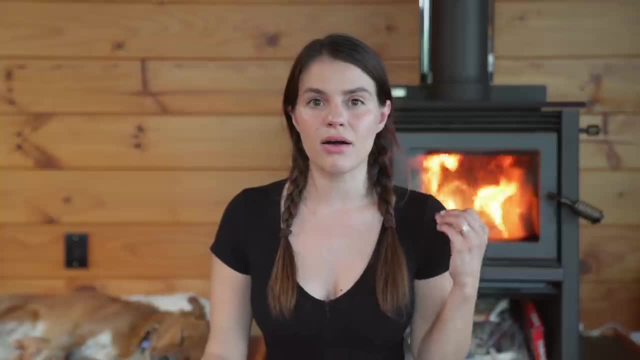 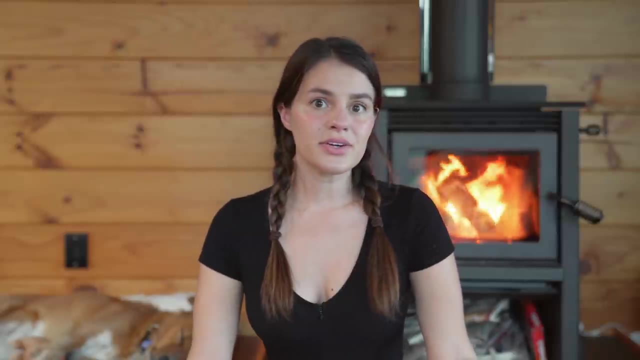 You can also find the recipe at my website, keriradcom. I'm pretty sure I have a blog post on exactly how to do that homemade pesticide there as well. Kale is easier to grow than your traditional regular, like romaine or butter lettuce. just because those are a little bit more fragile and finicky. They're really particular about the temperature outside. They love, like the spring time and maybe the early part of summer to mid. They can get a little bit too hot and they can get too cold, obviously. So they're a little bit more finicky but they're well worth putting them into your garden because obviously you can use lettuce for so many things And if you're gonna have all these wonderful veggies that are great for a fresh like yard to table salad. 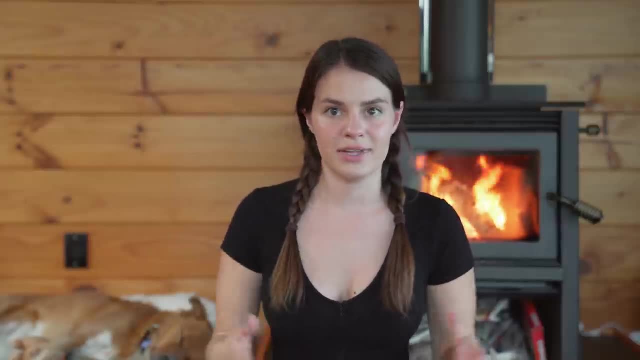 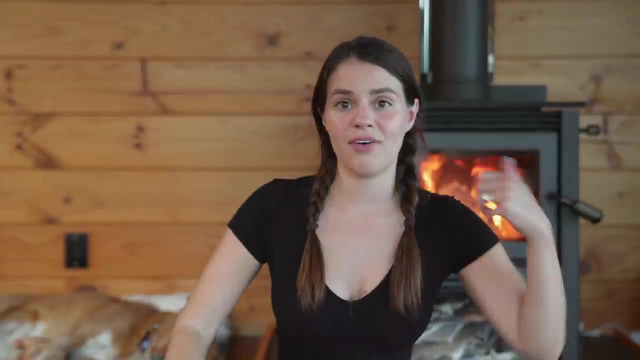 you gotta have some beautiful fresh leafy greens for that salad. My next recommendation are peppers. There are tons of different peppers that you can have growing in your garden. You can have jalapenos, you can have poblano, you can have regular chili. 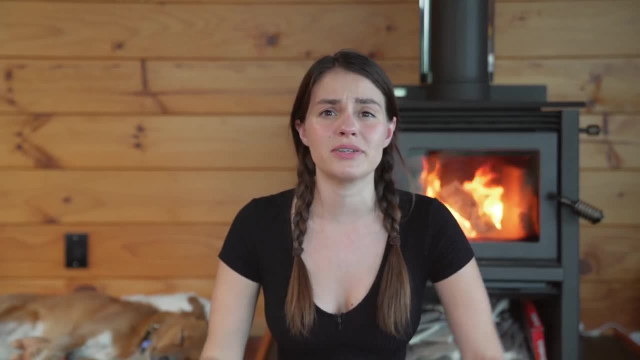 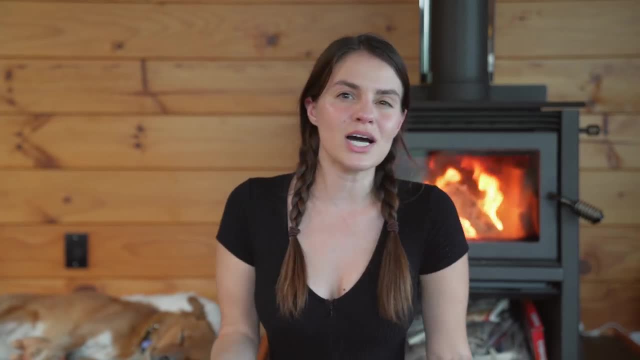 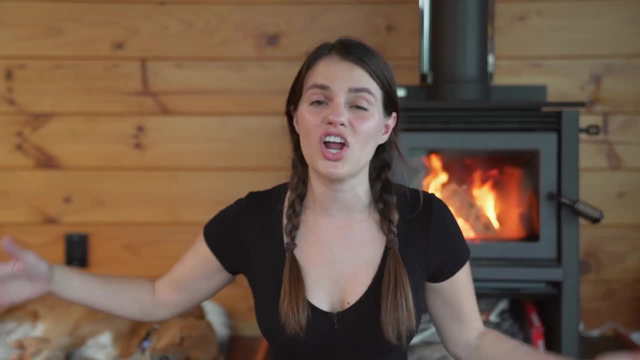 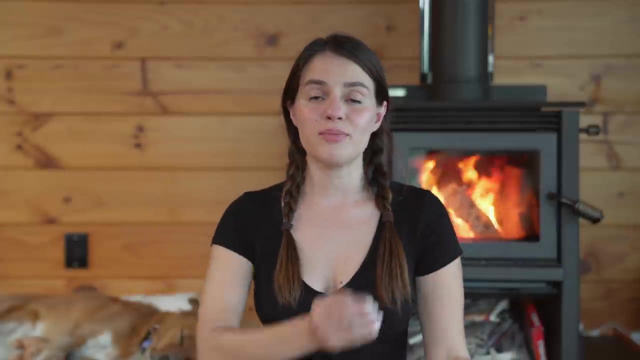 Also, the fun thing about peppers are that there are so many different options. There are so many different types of peppers and chilies to have in your garden. So how many you have in your garden probably just really depends on how much of a variety. 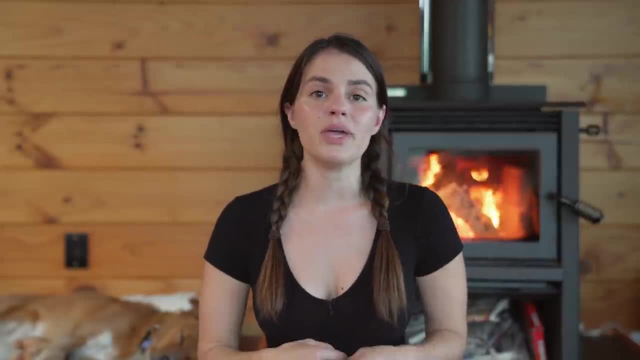 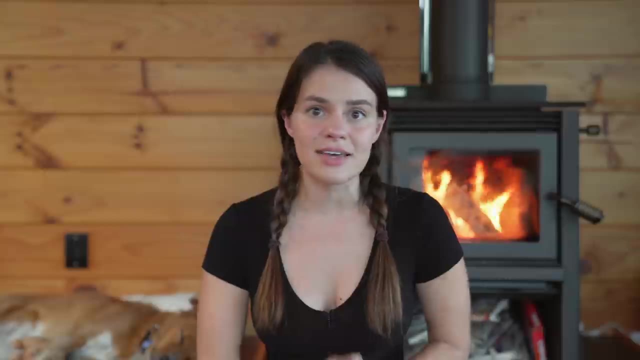 you want also how much you like spice. I know for us we loved having extra, because we would pull it off, we would bring it into the kitchen and we would create ground chili or chili flakes that you buy at the grocery store. and we didn't have to purchase that because we could make it at home. Speaking of a little bit of spice and a unique taste, I really love growing green onion or a spring onion in my garden. It's one of the first things that I planted. 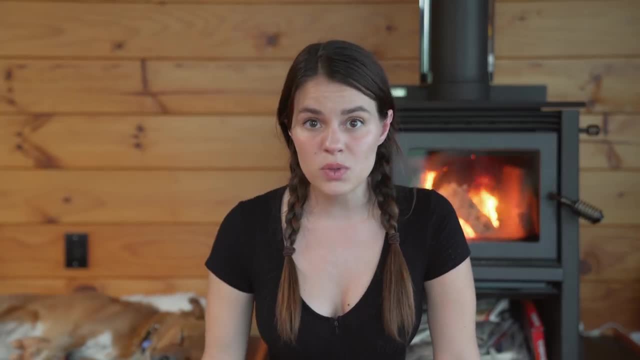 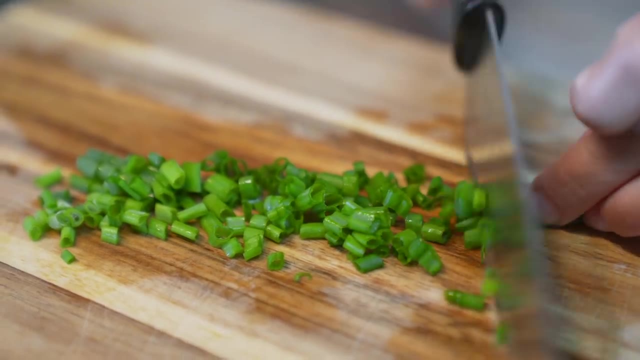 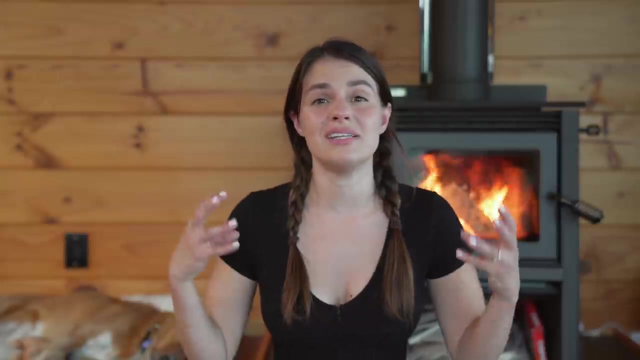 We probably use this vegetable the most when cooking because you can really put it on absolutely everything. Onion is more difficult to grow- just straight up onion- And a lot of people go for it right away. It takes longer to develop and it's actually quite fickle and difficult. 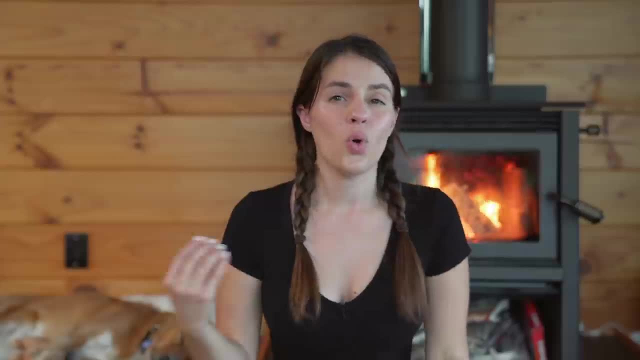 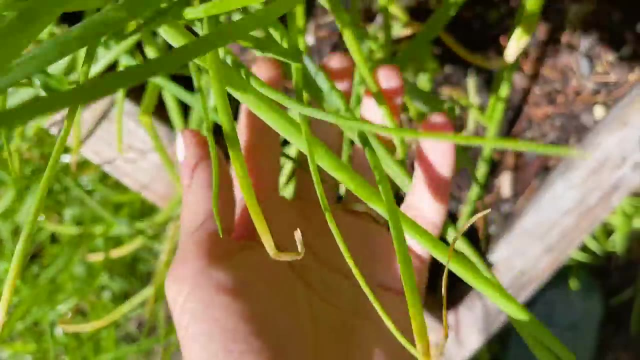 It really wants specific temperature, and we personally had a harder time growing onion. But when it came to spring onion or your green onion, it is extremely easy to grow. You can actually take the bulbs and you can grow it right in your kitchen. 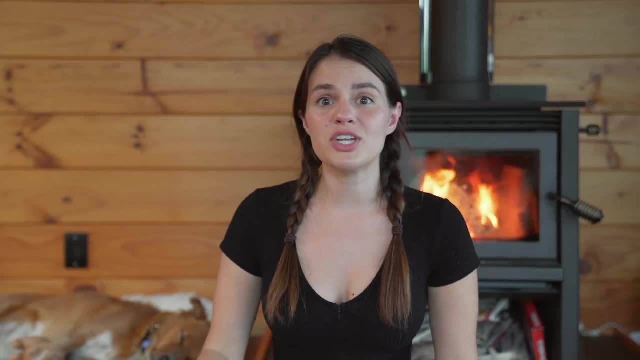 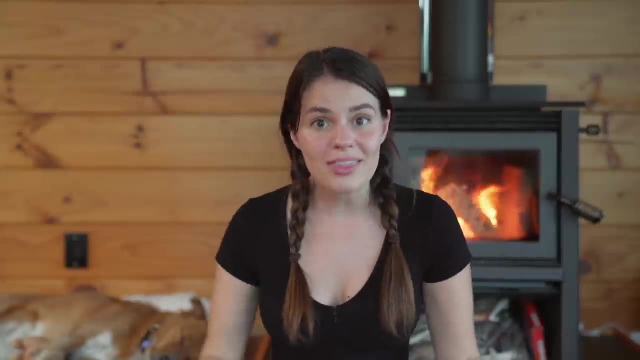 So if you don't have a vegetable garden, you have a couple of herbs on your windowsill. try taking the bulb of green onion, Putting it into some water, and it'll actually grow itself right there in your kitchen. And lastly but certainly not least, 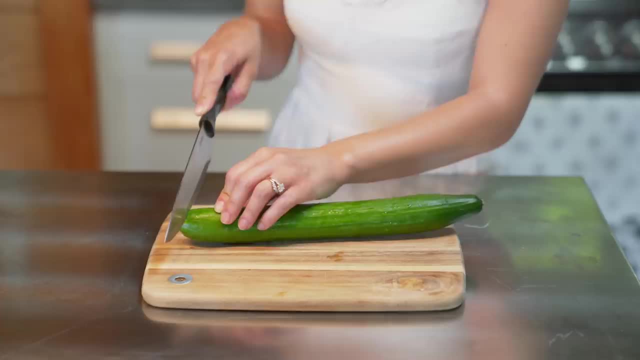 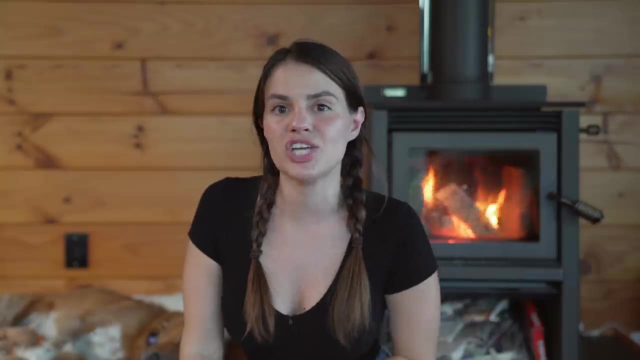 especially lately for me. I have been eating cucumber like crazy. I love it. Another one of those super juicy vegetables that when you bring them into the kitchen from the garden and you cut one open and you're just like I created this juice with the water. 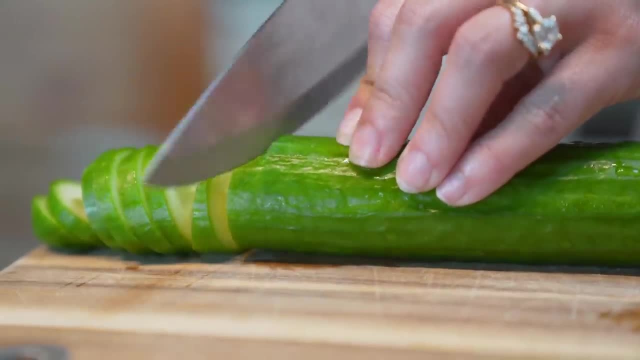 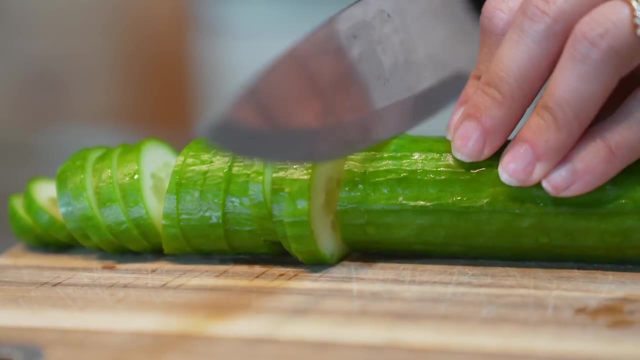 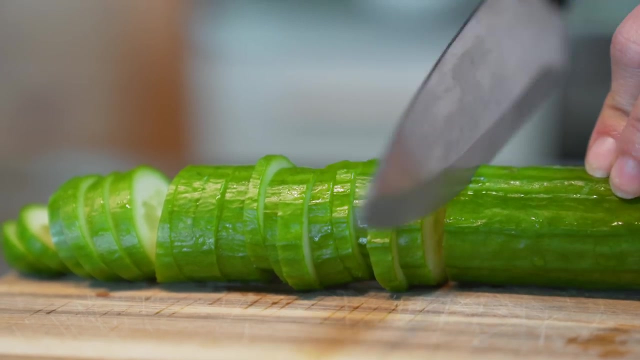 I've been giving these plants and it's just a beautiful, beautiful, beautiful day, beautiful vegetable, and it's so fresh and it can go into so many things that instantly make whatever dish you're putting it into even more fresh. I love doing a cucumber and tomato salad. 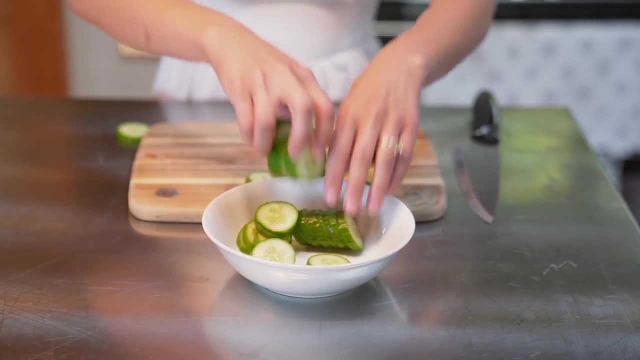 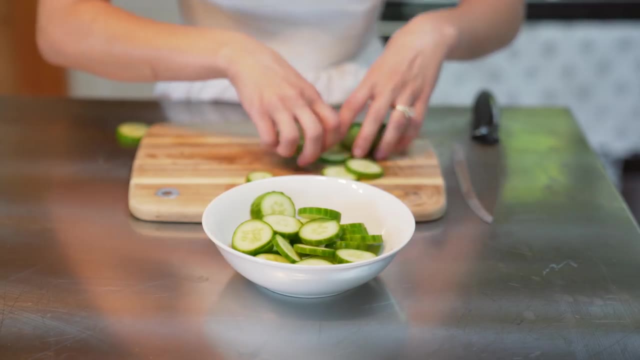 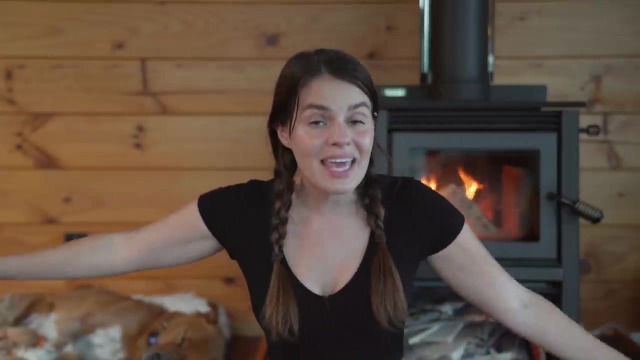 just super simple with some feta. I love putting cucumber into any Mediterranean dish, Like if I'm doing a Mediterranean chicken with some yogurt and a wrap. I love having cucumber as an option there. Cucumber is another one of those plants where it grows quite abundantly and quite big. 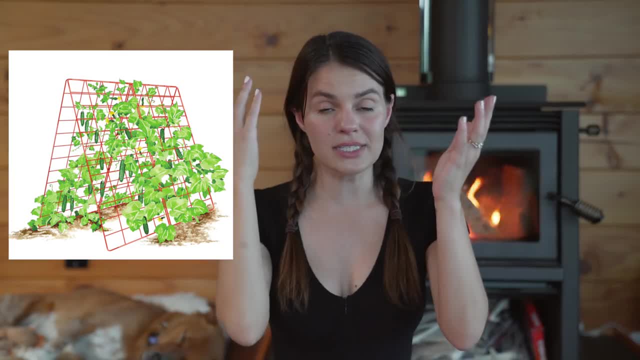 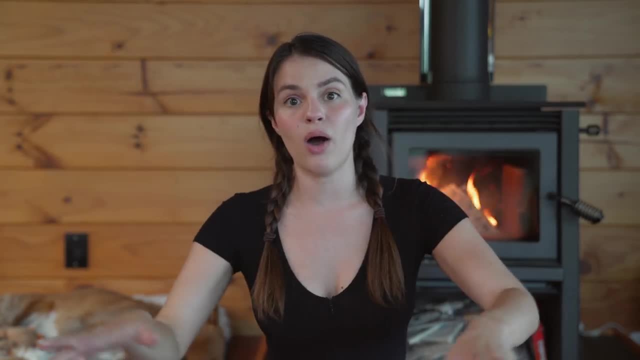 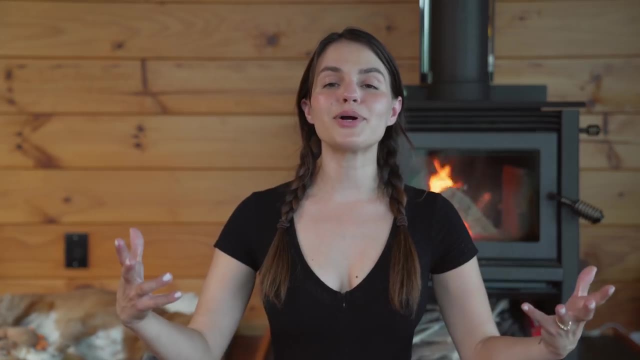 It's like a big vine plant and it likes to grow upwards, So you'll want to have some sort of trellis above your cucumber. If you let it just kind of grow outwards in your garden, it will probably rot and it won't grow the best. Zucchini and cucumber are companion plants and 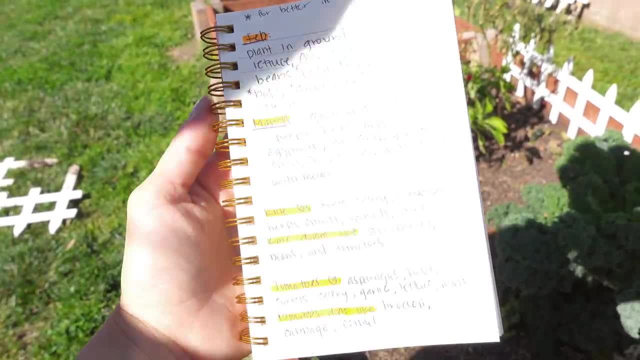 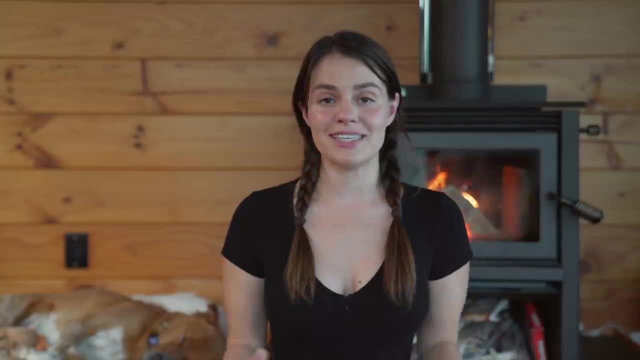 companion plants are actual vegetables that like to grow near each other In the garden and, like I said in my how to build a vegetable garden video, veggies can be quite like humans. There are specific people that they like or veggies that they like being near, and that 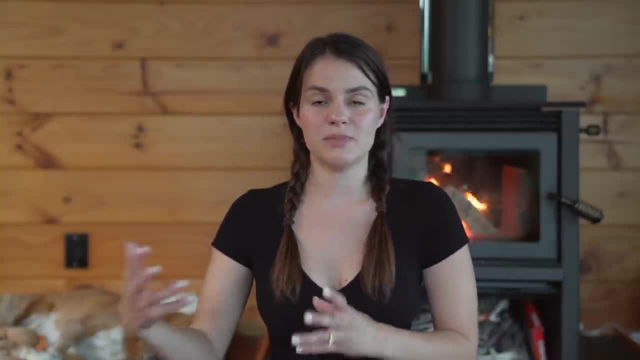 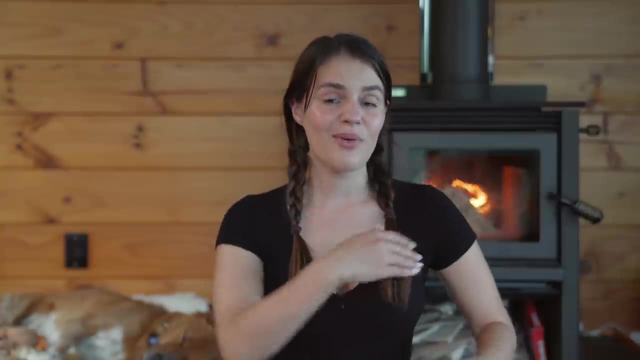 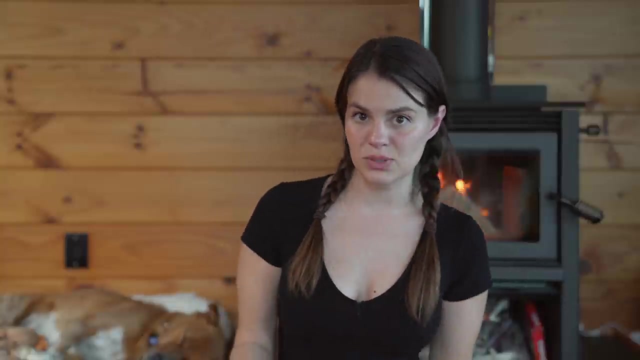 they grow better when they are near this specific person. And then there are some plants that are not good for them, just like toxic people for humans, where we aren't doing our best when we are around them. Basil and tomato, for example. they love being next to each other. They love 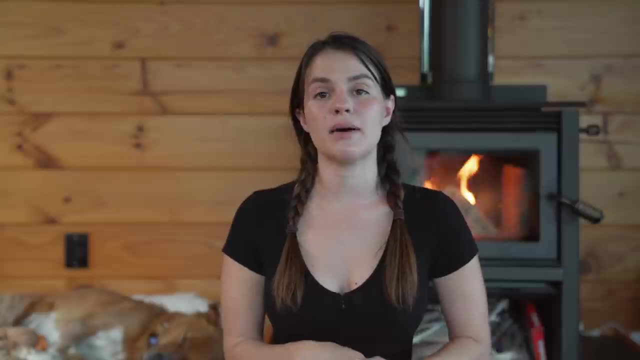 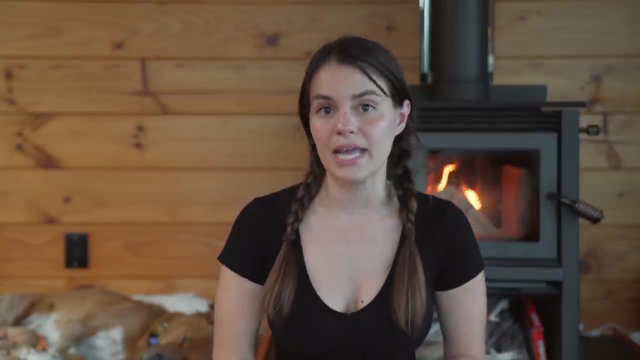 being next to each other in the garden. Basil actually protects tomato in some ways from different pests that really love that beautiful juicy fruit coming off of the plant. If you plan on growing both zucchini and cucumber, then maybe find a place in your garden where they both have.